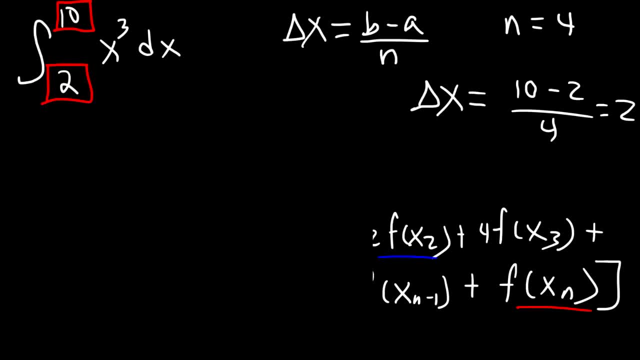 Now let's create a number line. So because n is 4, there's going to be 4 subintervals but 5 points, and you can see delta x is 2 here. Now for the Simpson's rule and the trapezoidal rule, we're going to use all 5 points. 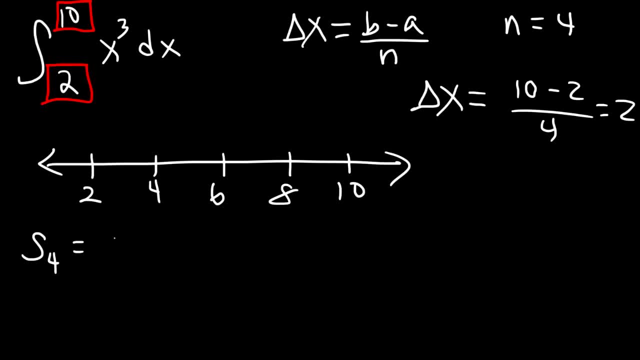 So it's going to be s sub 4, and that's equal to delta x, which is 2, divided by 3, and it's going to be f of 2 plus 4 times f of 4, plus 2 times f of 6, plus 4 times f of 8,. 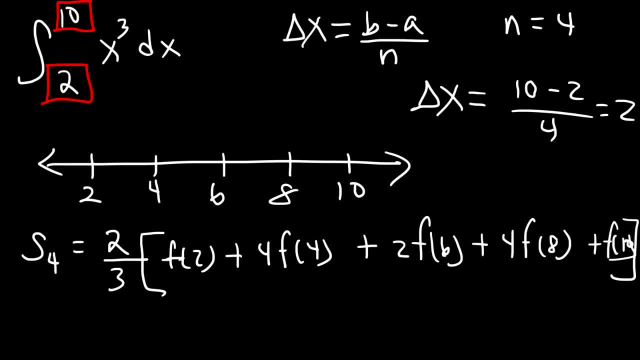 and then plus f of 10.. Now keep in mind: f of x is x cubed. Okay, Okay, Okay, Okay, Okay, Okay, Okay. So 2 to the 3rd power is 8.. 4 to the 3rd power, that's 64.. 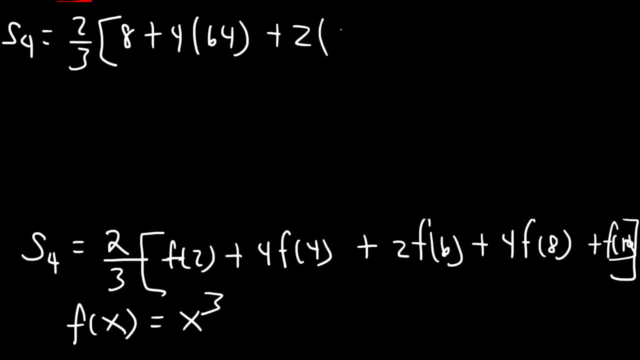 And then 6 to the 3rd power, that's 216.. 8 to the 3rd power: I've got to type that one in, So that's going to be 512.. And then 10 to the 3rd is 1000.. 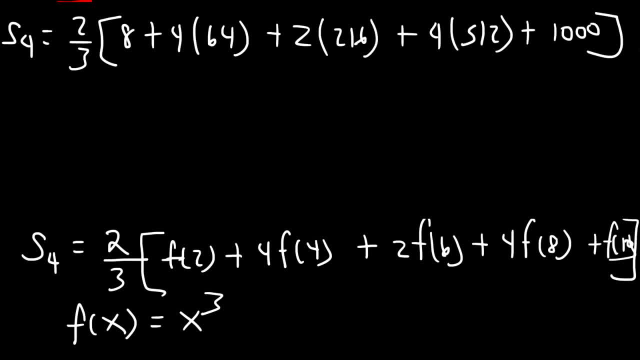 So go ahead and type in what you see. So the value I got is 2,496.. Now let's calculate the value of the definite integral using integration. So let's integrate x cubed dx from 2 to 10.. The antiderivative of x cubed is x to the 4th divided by 4.. 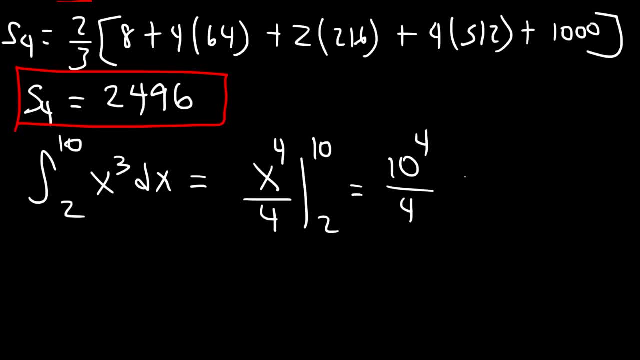 And if we plug in 10, it's going to be 10 raised to the 4th over 4, and then minus 2 raised to the 4 over 4.. So 10 to the 4th power. 10 times 10 is 100, times another 10, that's 1,000, times 10,. 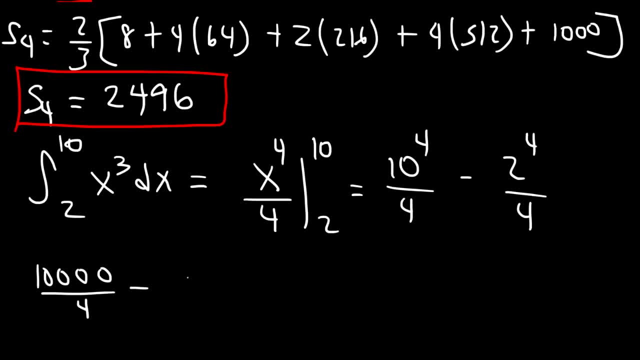 that's 10,000.. 2 to the 4,, that's 1,000.. 2 to the 4,, 2 times 2 times 2 times 2, that's 16.. 10,000 divided by 4 is 2,500.. 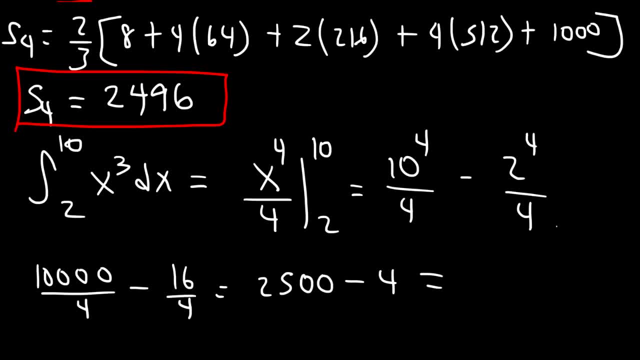 16 divided by 4 is 4.. And 2,500 divided by 4 is 2,496.. Now this is one of those rare cases where these two answers are the same, But in other cases you'll find that the Simpson's rule is a very good approximation. 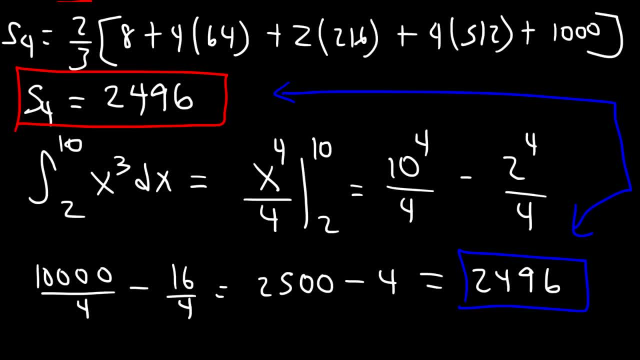 of the value of the definite integral, So you can use it to estimate the integral, Or you can just make the area under a curve Or evaluate a definite integral if you're given a problem with a data table, And so that's it for this particular problem. 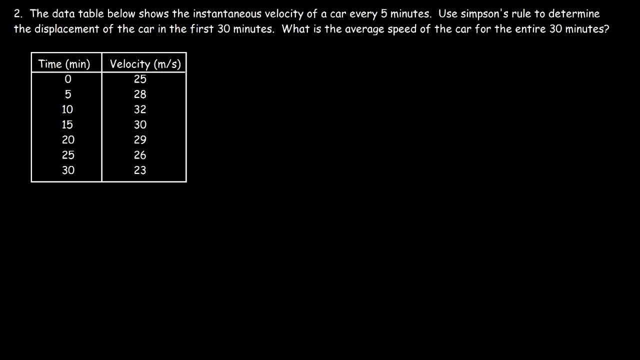 Now let's work on this word problem. The data table below shows the instantaneous velocity of a car every 5 minutes. Use Simpson's rule to determine the displacement of the car in the first 30 minutes And also determine the average speed of the car for the entire trip. 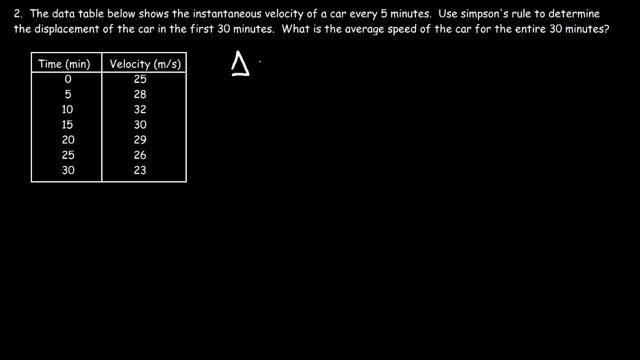 So first we need to calculate delta x. So that's going to be b minus a divided by n. So what's a and b in this problem? Well, the interval is the first 30 minutes, so a is 0, b is 30. 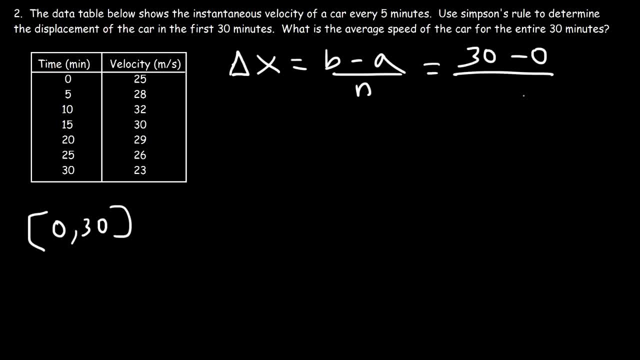 So it's going to be 30 minus 0, and then what is n in this problem? Well, n is the number of intervals. this is going to be one interval, and then 2,, 3,, 4,, 5,, 6.. 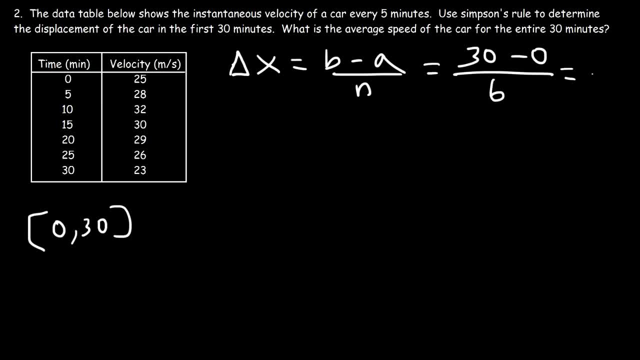 So n is 6. And 30 divided by 6 is 5. And we can see that it's spaced out 5 minutes every time the velocity is being measured. Now notice that the velocity is in meters per second and the time is in minutes. 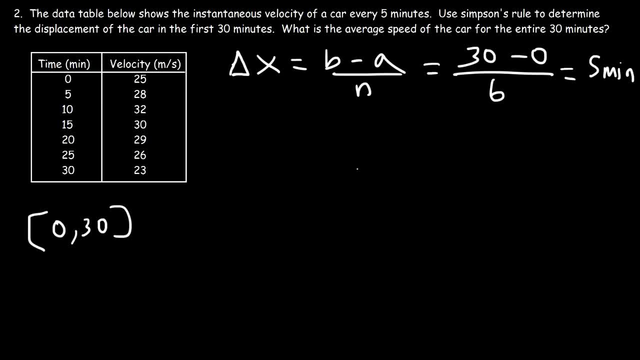 So we need to convert delta x from being in minutes to seconds, And 1 minute is 60 seconds. So 5 minutes is going to be 5 times 60, which is 300.. So that's what we're going to use for delta x. 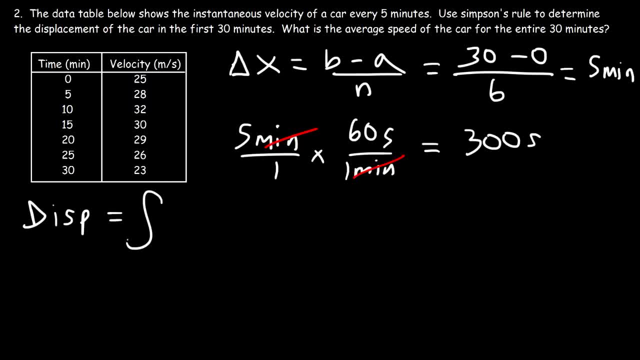 Now you need to know that the displacement is going to be the definite integral from a to b of the velocity function. So we can estimate that definite integral using Simpson's rule, in this case with 6 subintervals. So n is 6.. 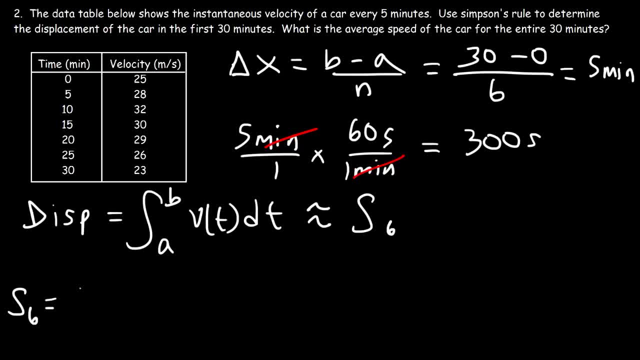 So s of 6 is going to be delta x, which is 300 seconds divided by 3, and then the first point is going to be f of 0, and then it's going to be 4 times f of 5.. 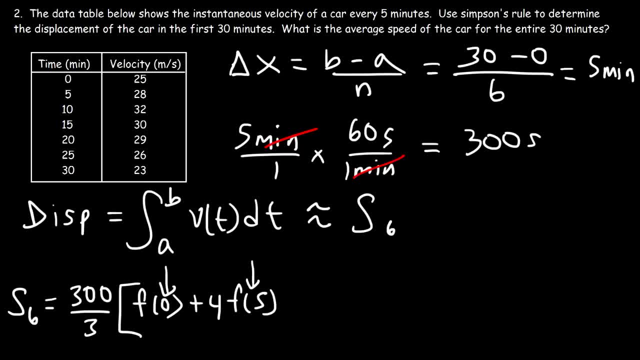 Now keep in mind These values. that's basically the time in minutes, But the y value that it corresponds to is going to be in meters per second, which will cancel with the 300 seconds, So it's going to work out this way. 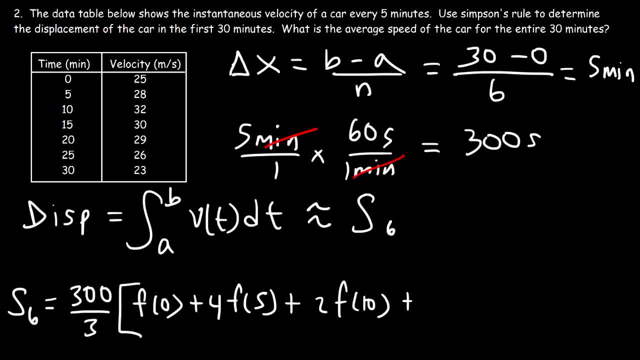 And then it's going to be 2 times f of 10 plus 4 times f of 15, and then 2 times f of 20 plus 4 times f of 15.. So that's going to be the time in minutes. 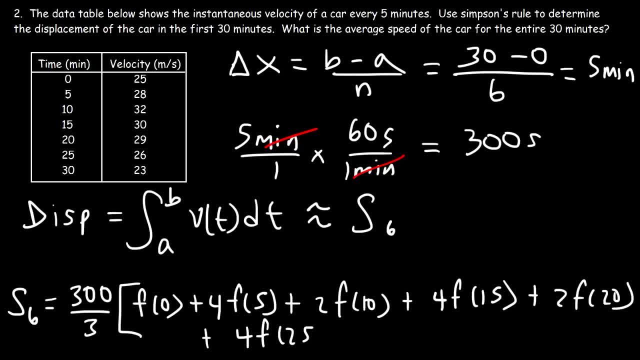 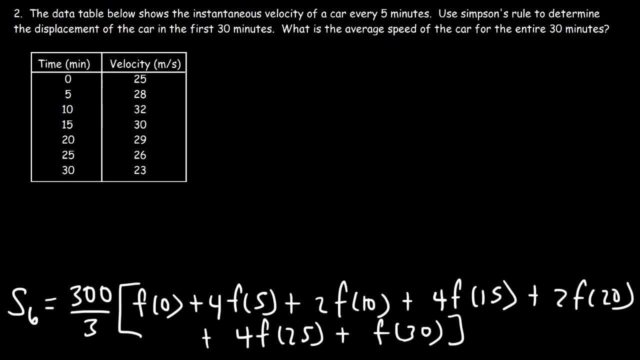 This is 4 times f of 25, and then the last one is just going to figure out the term there, which is 2 times f of 16.. 3 times f of 27 plus f of 30.. Now it's actually no 1's and 2's. 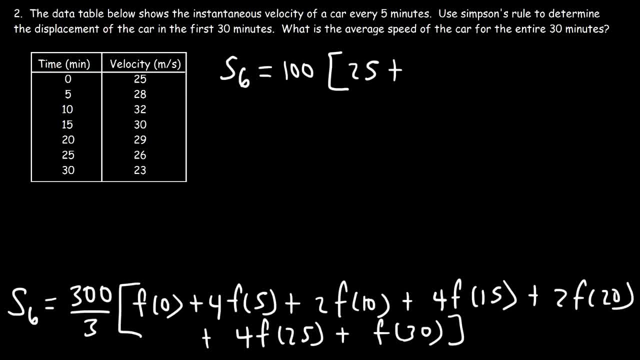 This is just anotherыс puedanstoff, some time in third order. And then we need to find the god's speed s, which is 1 second and explicit 4 times f of 1 Electron times repeatedly finished second. So we're going to-so in this case, what do I have here? 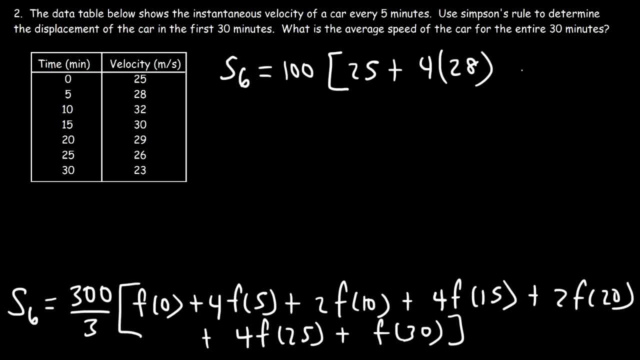 4 times f of 25, and then the last one is just going to be f of 30.. F of 5, which is 28, and then 2 times F of 10, that's 32, and then 4 times F of 15. 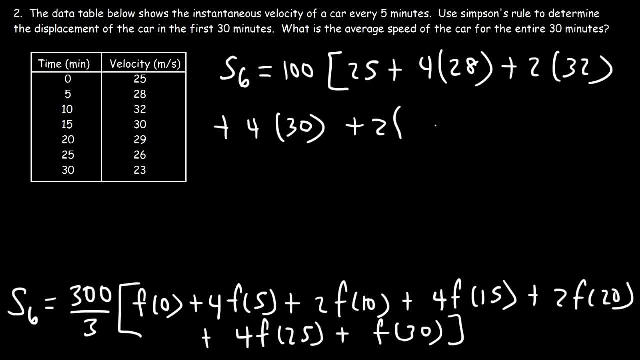 which is 30, and then 2 times F of 20, that's 29, plus 4 times F of 25, which is 26, and then F of 30 is 23, based on the table. so this is equal to 100 and then. 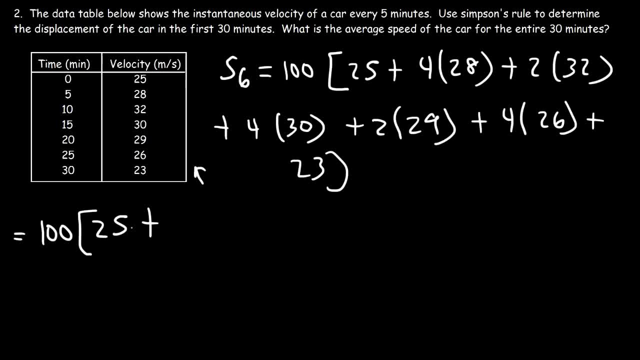 4 times 28, that's 112. 2 times 32 is 64, 4 times 30 is 120. 2 times 29 is 58. 4 times 26 is 27, and then 4 times 28 is 28, and then 4 times 28 is 28 and then 4 times. 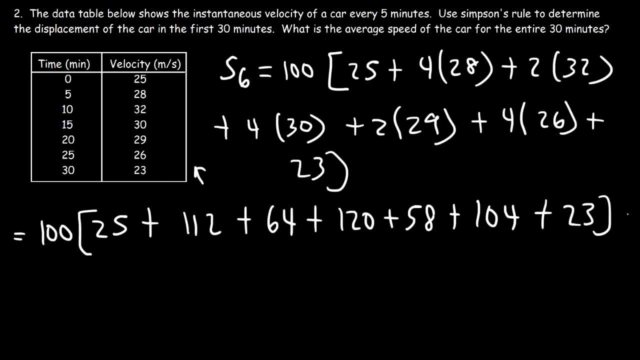 26 is 24 and then plus 23. so let's just go ahead and plug this in to a calculator and get the final answer. so S of 6 is going to be 50,600 meters. so that's the displacement of the vehicle in the first 30 minutes. if you want to convert that to: 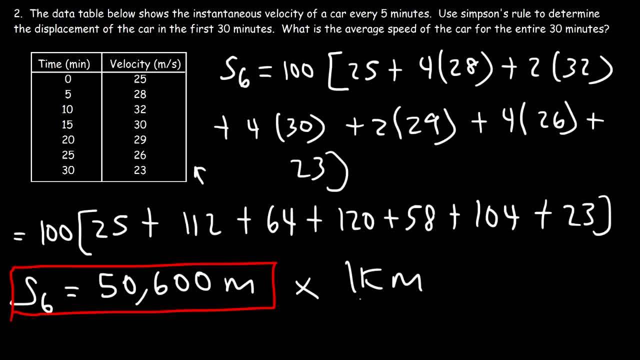 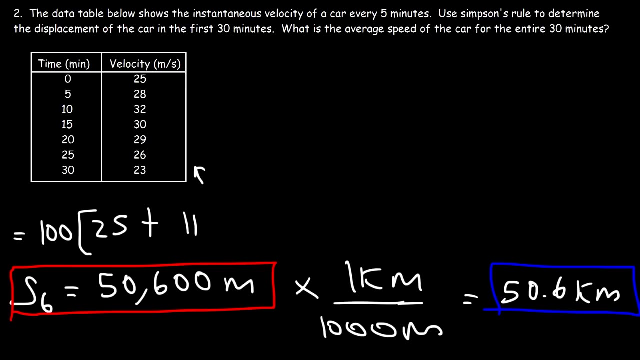 kilometers. simply divide by a thousand. a thousand meters equals one kilometer, so this is about fifty point six kilometers. now let's calculate the average speed of the car for the entire 30 minutes. the total distance that the car travels is going to be fifty thousand six hundred. 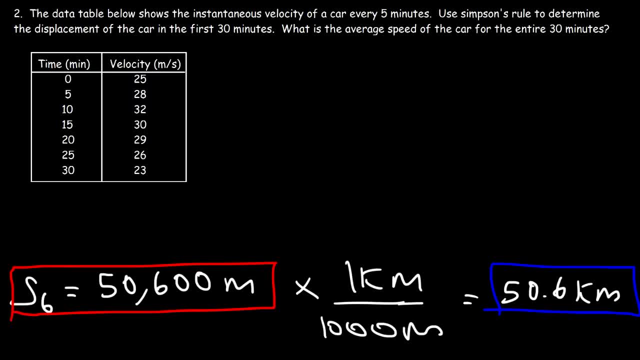 unless the car changes direction, which we have no indication that it changed direction- the velocity is positive. if the car stayed in one direction, the displacement and the total distance will be the same. if the car changes direction, displacement and distance will not be the same. now, average speed is equal to: 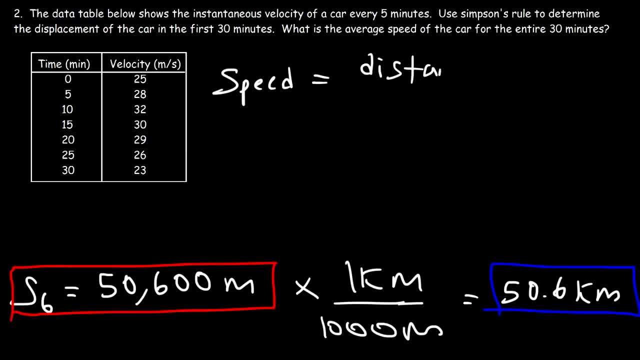 the total distance traveled divided by the total time, and so the total distance traveled is 50,600 meters and the time is 30 minutes. but we need to get that in seconds, so we need to multiply 30 minutes by 60 seconds per minute, so 30.